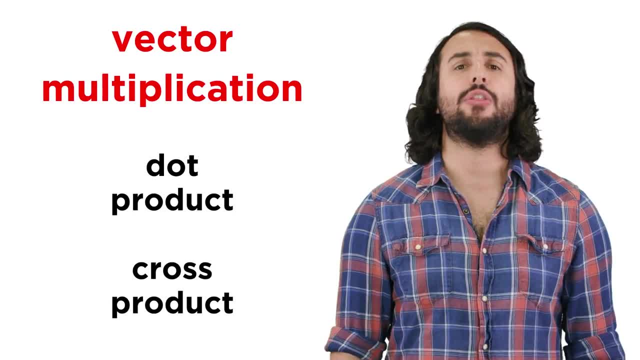 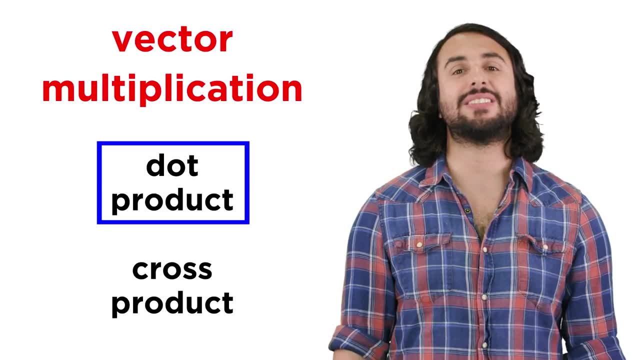 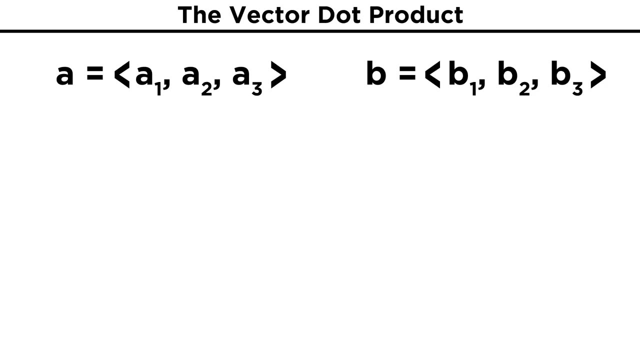 because we have to understand what we mean by this operation. There are actually two different ways that we can multiply two vectors, and the first kind of multiplication will give us something called the dot product. Let's learn how to perform this operation. The dot product is fairly intuitive. 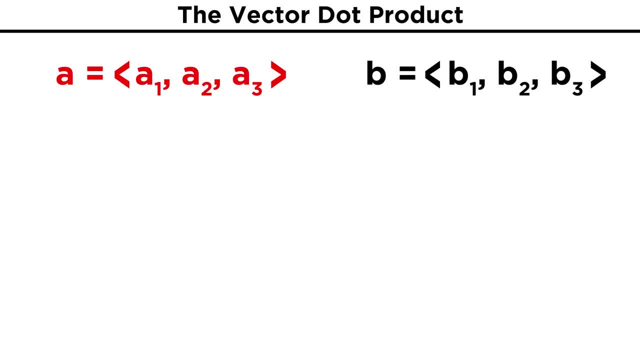 If we have some vector A with components A1,, A2, and A3, and another vector B with components B1,, B2, and B3,, then its dot product will be denoted this way: as A dot B, This will be equal to A1B1, plus A2B2, plus A3B3. 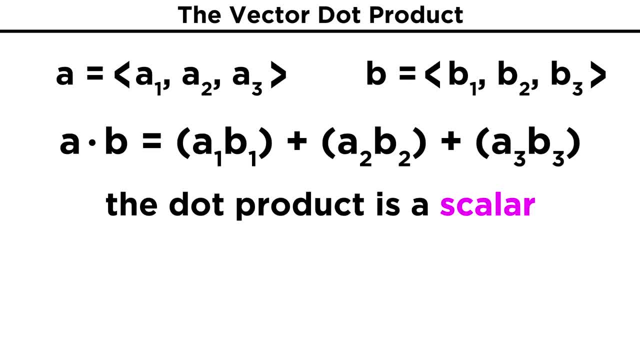 It is very important to note that this is a scalar product. The dot product does not give us another vector. It takes two vectors as an input and gives us one number as an output. For example, if A is two four and B is one negative three, then A dot B is equal to two. 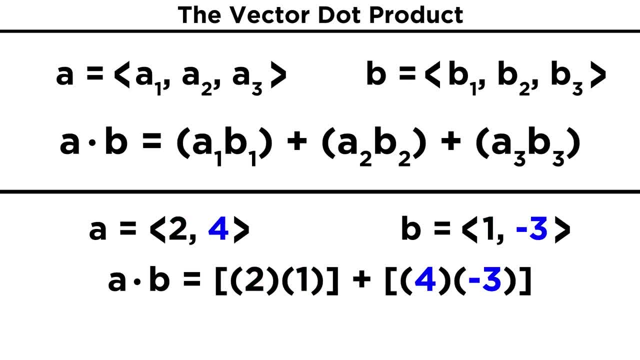 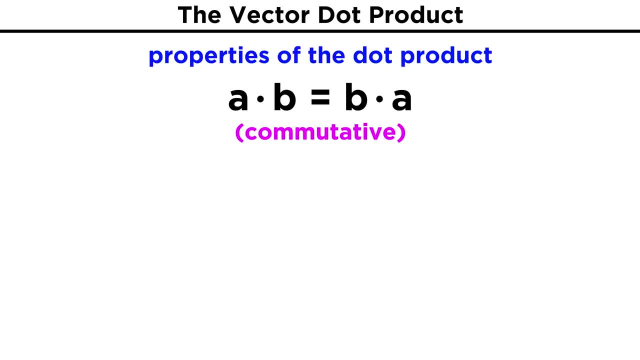 B2, and B3. It is equal to two times one plus four, times negative three, or two minus twelve, which gives us negative ten. Because the dot product involves simple multiplication, it has very intuitive properties: A dot B equals B dot A, because it doesn't matter what order in which numbers are multiplied. 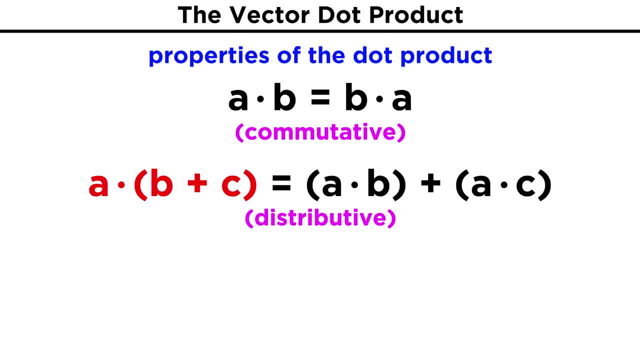 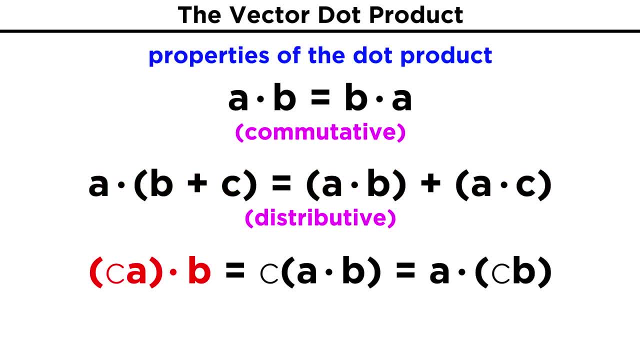 as A dot B plus A dot C. A scalar times a vector involved in a dot product is the same as the scalar multiplied by the dot product or the other combination of scalar and vector involved in the same dot product. A dot A is simply the length of A quantity squared. 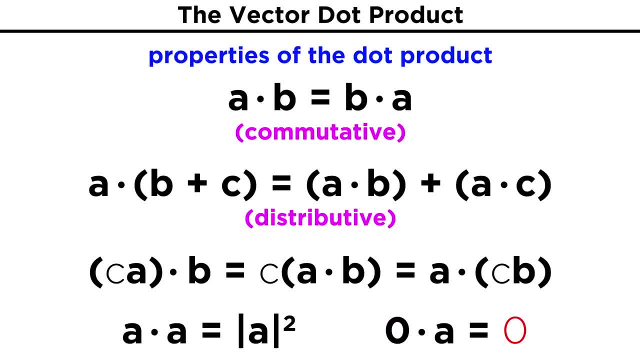 And the zero vector, dot. A, is the number you multiply based on the number of North and South zero, because we are just multiplying each component of A by each component of the zero vector, which are all zeros, and then adding all of those zeros up to get zero. 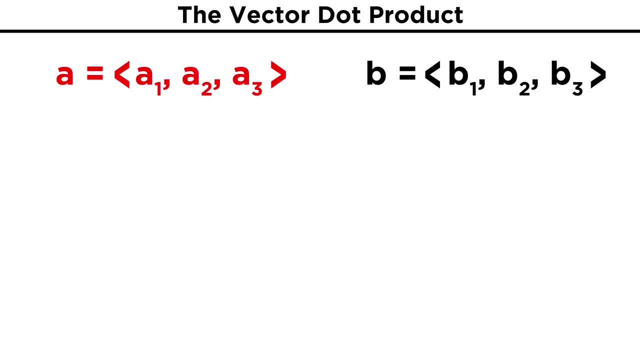 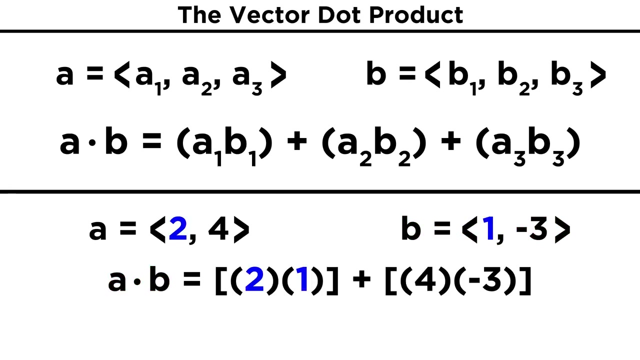 If we have some vector A with components A1, A2, and A3, and another vector B with components B1, B2, and B3, then its dot product will be denoted this way, as A dot B. This will be equal to A1B1, plus A2B2, plus A3B3. It is very important to note that this is a scalar product. The dot product does not give us another vector. It takes two vectors as an input, and gives us one number as an output. For example, if A is two, four, and B is one, negative three, then A dot B is equal to two, B2, and B3. It is equal to two times one, plus four times negative three, or two minus twelve, which gives us negative ten. 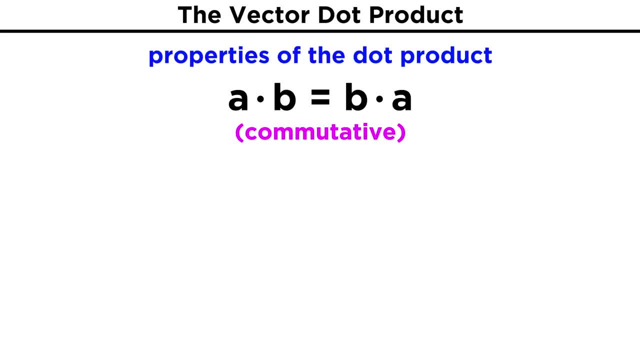 Because the dot product involves simple multiplication, it has very intuitive properties. A dot B equals B dot A, because it doesn't matter what order in which numbers are multiplied. The distributive property also holds, and A dot the sum of B is equal to B dot A. A dot is the sum of B and C, or A dot the vector that results from adding B and C, is the same as A dot B plus A dot C. A scalar times a vector involved in a dot product is the same as the scalar multiplied by the dot product, or the other combination of scalar and vector involved in the same dot product. 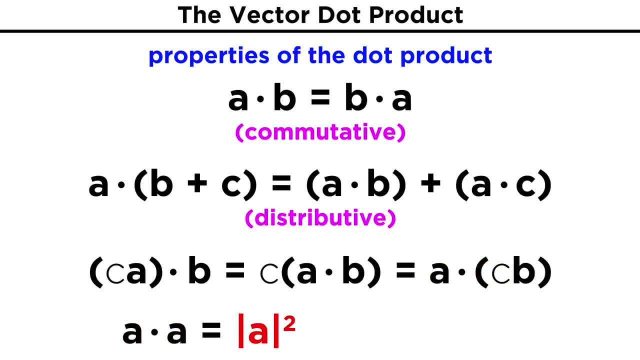 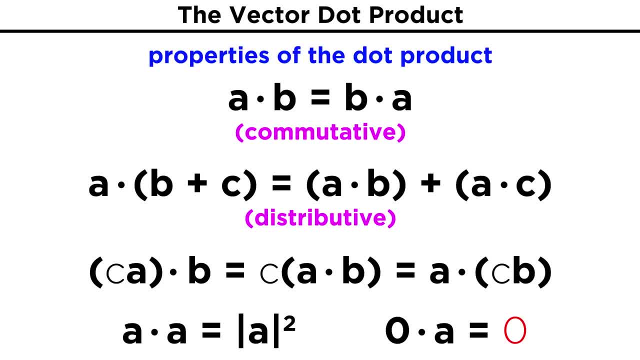 zero, because we are just multiplying each component of A by each component of the zero vector, which are all zeros, and then adding all of those zeros up to get zero. 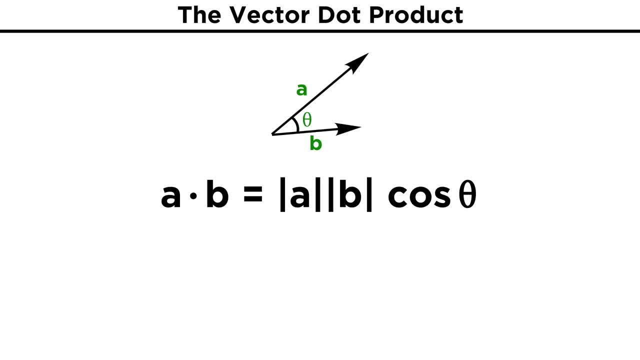 The dot product also crops up in an interesting theorem, which says that for two vectors, A and B, A dot B is equal to the length of A times the length of B times the cosine of the angle between them. 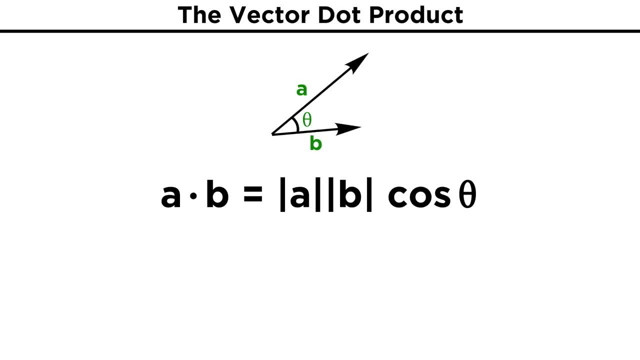 The dot product also crops up in an interesting theorem which says that for two vectors, A and B, A dot B is equal to the length of A times the length of B times the cosine of the angle between them. This means that if we want to calculate the angle between two vectors, we can simply bring 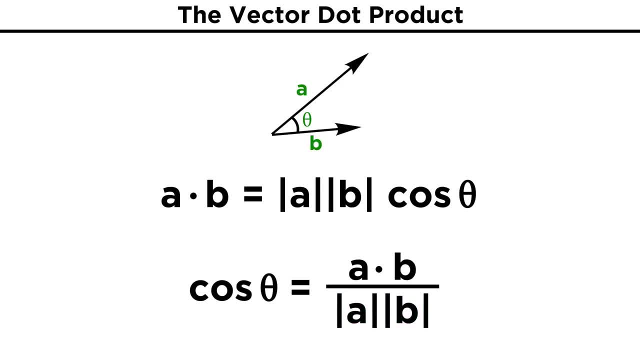 these vector lengths to the other side of the equation and we get cosine theta as being equal to A dot B divided by the product of the vector lengths. This is one of the reasons the dot product is useful, as it gives us a great way to calculate. 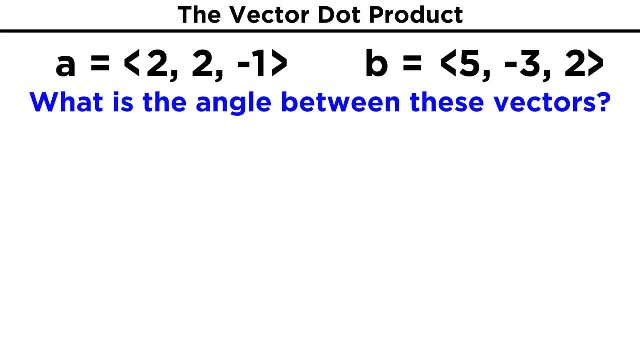 angles without doing any trigonometry. Let's give it a try. What is the angle between vector A with components A and B? Let's try it Well. first let's find the length of each vector. For A, that's two squared plus two squared plus negative, one squared, all under a square. 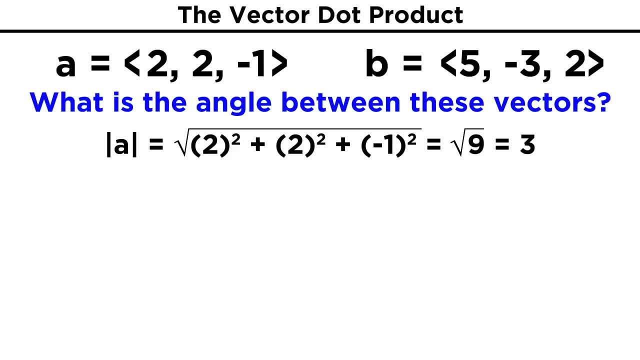 root. We simplify to get nine and then take the square root to get three For B, we get five squared plus negative three squared plus two squared under the square root. We simplify to get thirty-eight And we can just leave this as root: thirty-eight. 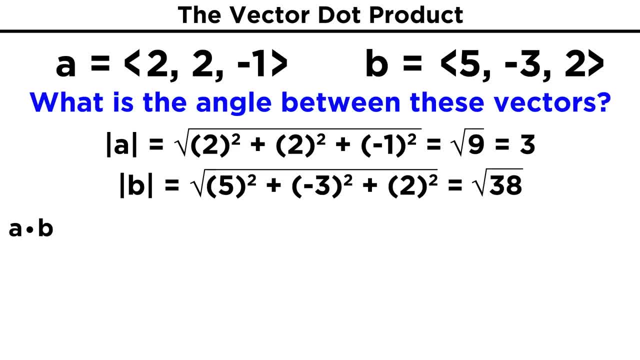 Now let's perform the dot product. Multiplying the corresponding components, we get two times five plus two times negative. three plus negative one times two. That's ten minus six minus two or two. So plugging everything in, we get two on the top and then three times root thirty-eight. 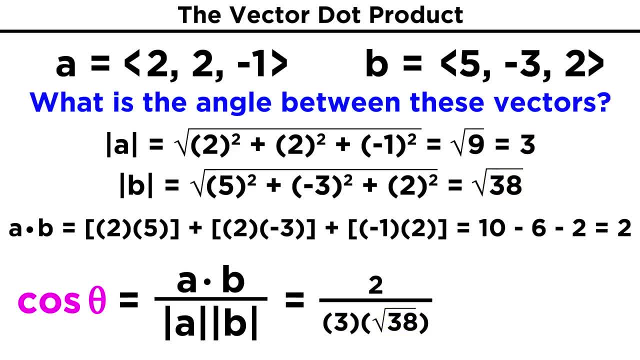 That is equal to the cosine of A. Now let's look at the cosine of the angle between the vectors. To solve for the angle we just take the inverse cosine and since this is a pretty ugly number, we just plug it into a calculator to get some decimal and press the inverse cosine button. 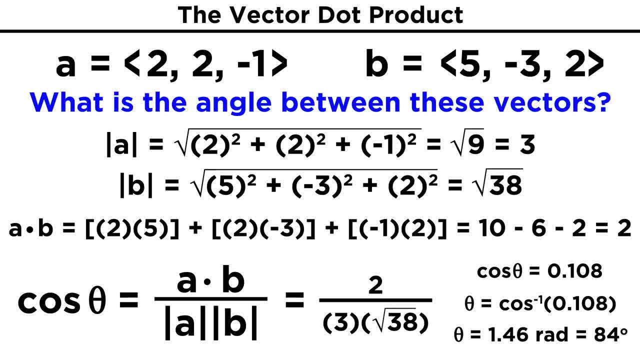 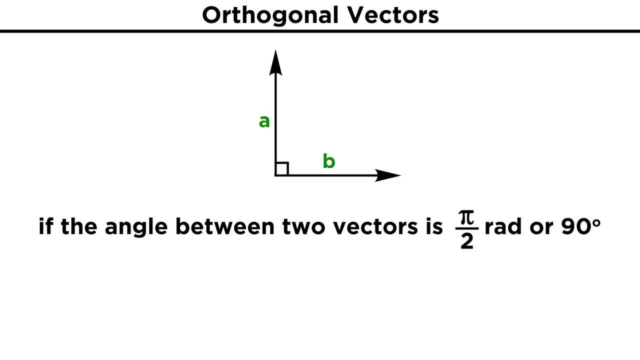 That gives us around one point four six radians, which is about eighty-four degrees. This operation leads us to another definition. We want to understand that if the angle between two vectors is half pi radians or half pi radians or ninety degrees, these vectors are orthogonal. 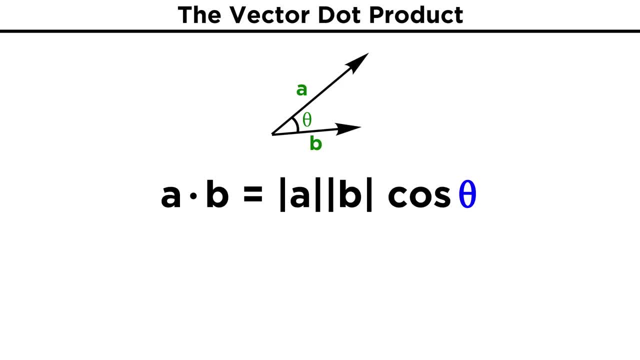 This means that if we want to calculate the angle between two vectors, we can simply bring these vector lengths to the other side of the equation, and we get cosine theta as being equal to A dot B divided by the product of the vector lengths. 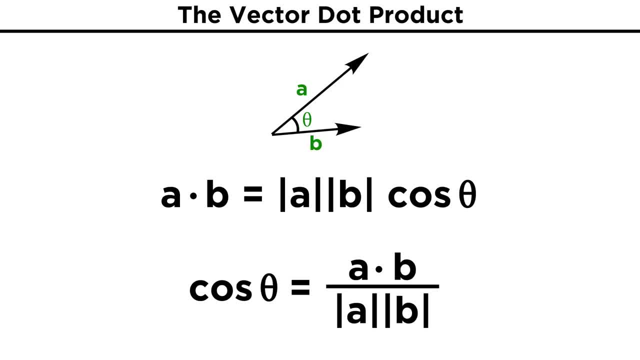 This is one of the reasons the dot product is useful, as it gives us a great way to calculate angles without doing any trigonometry. 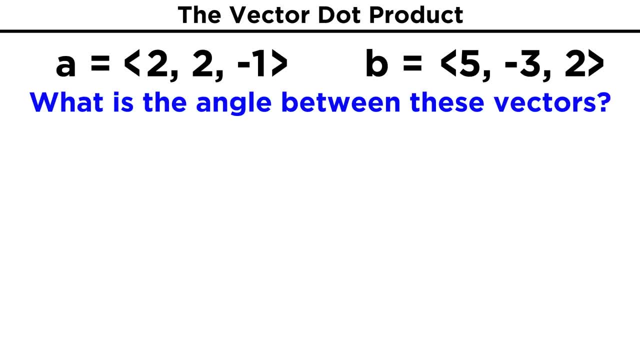 Let's give it a try. What is the angle between vector A with components A and B? Let's try it. 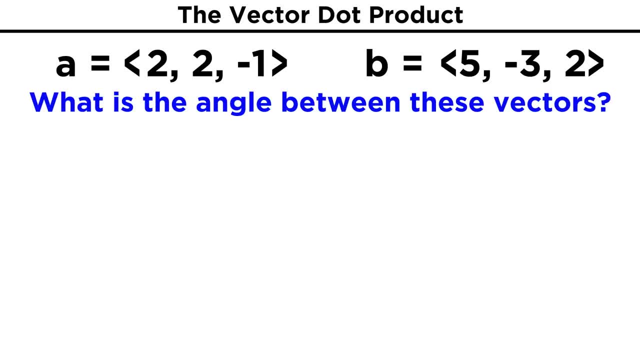 Well first, let's find the length of each vector. 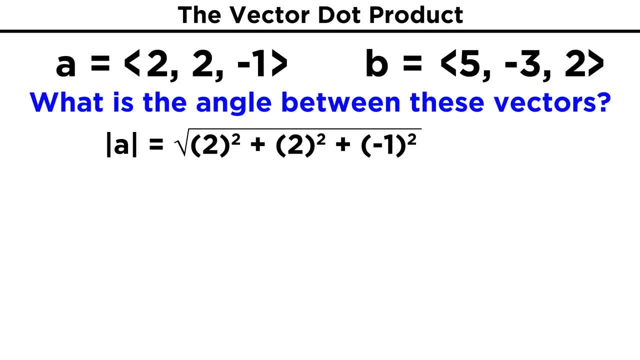 For A, that's two squared, plus two squared, plus negative one squared, all under a square root. 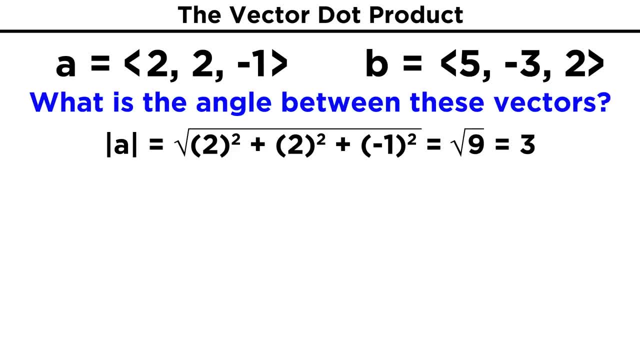 We simplify to get nine, and then take the square root to get three. 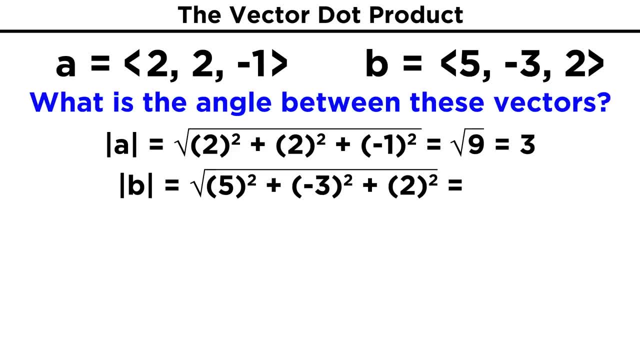 For B, we get five squared, plus negative three squared, plus two squared, under the square root. 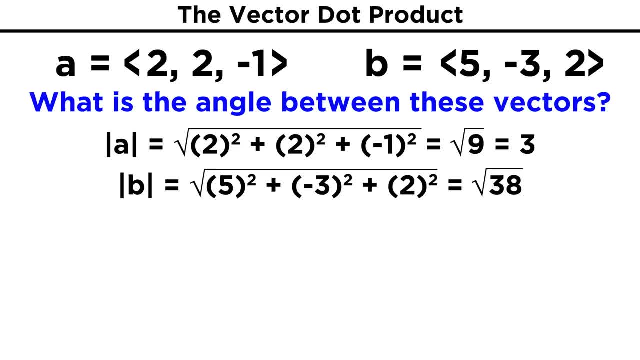 We simplify to get thirty-eight. And we can just leave this as root thirty-eight. 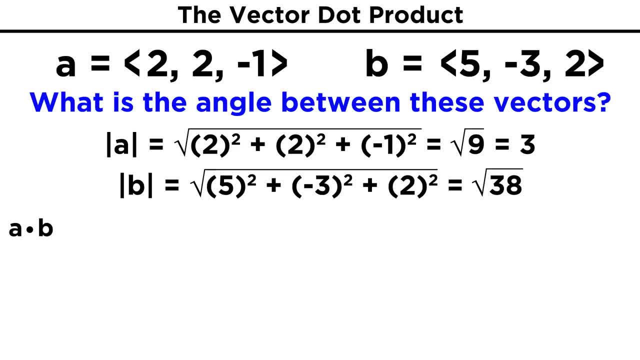 Now let's perform the dot product. Multiplying the corresponding components, we get two times five, plus two times negative three, plus negative one times two. 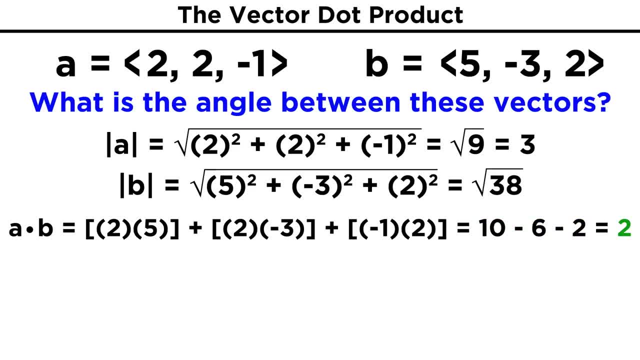 That's ten minus six minus two, or two. 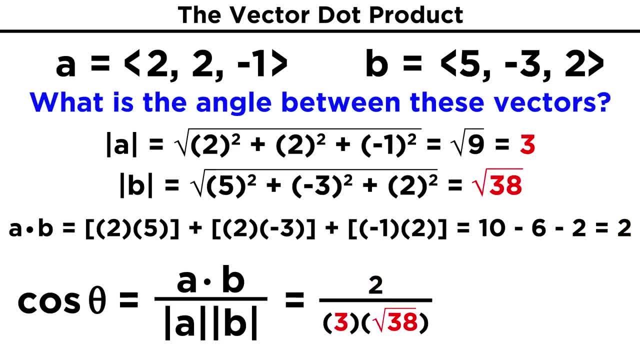 So plugging everything in, we get two on the top, and then three times root thirty-eight. That is equal to the cosine of A. 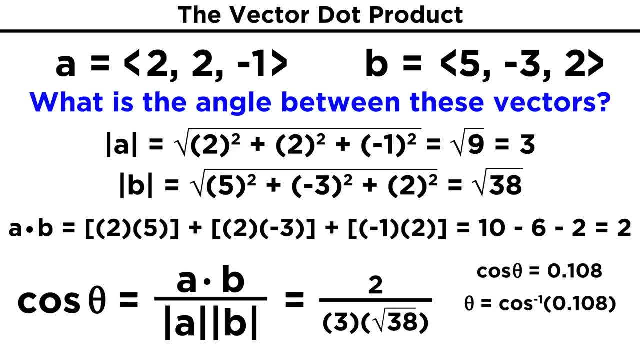 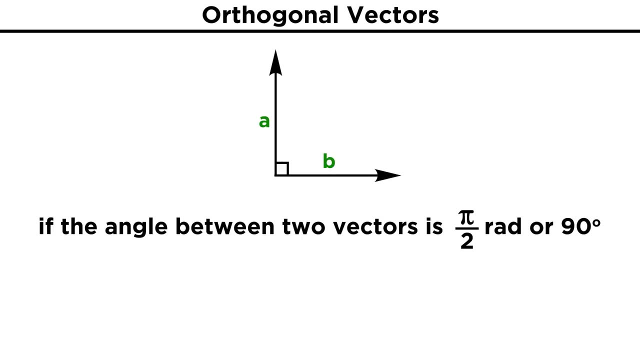 Now let's look at the cosine of the angle between the vectors. To solve for the angle, we just take the inverse cosine, and since this is a pretty ugly number, we just plug it into a calculator to get some decimal, and press the inverse cosine button. That gives us around one point four six radians, which is about eighty-four degrees. This operation leads us to another definition. We want to understand that if the angle between two vectors is half pi radians, we're going to get zero.